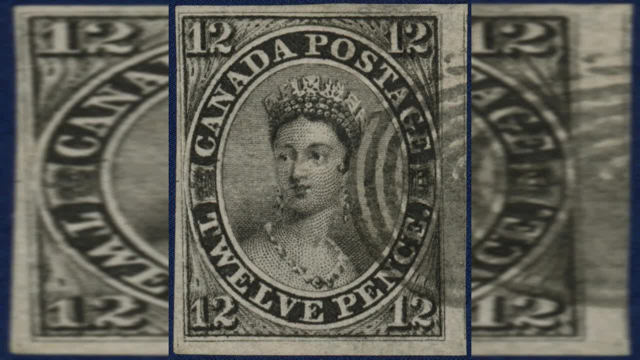 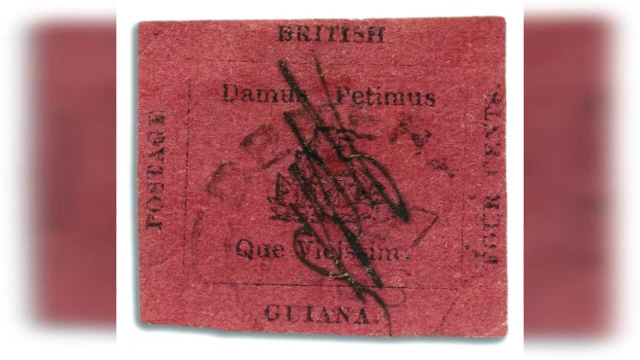 The 12 pence black is one of Canada's earliest stamps, issued in 1851.. It features a portrait of Queen Victoria and was used for domestic and international postage- Number 16.. British Guiana 4C cotton reels 1852, estimated value: $600,000. 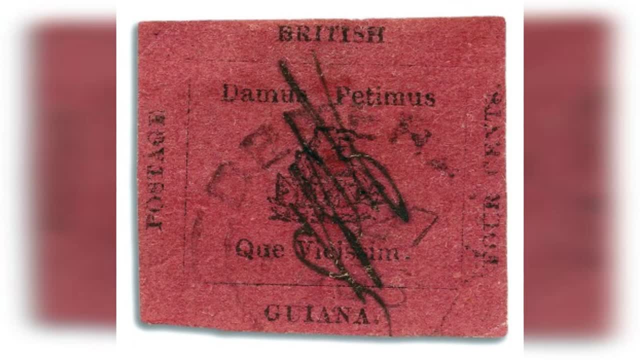 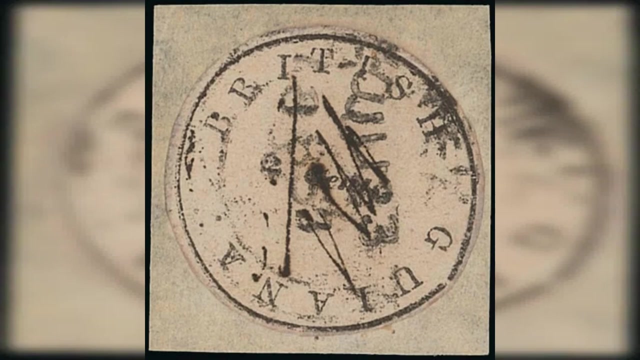 As previously mentioned, the British Guiana 1C magenta is one of the most famous and valuable stamps in the world. It was issued in British Guiana- now Guyana- when a shipment of postage stamps from England was delayed In 2014,. it was sold for a record-breaking $9.5 million. 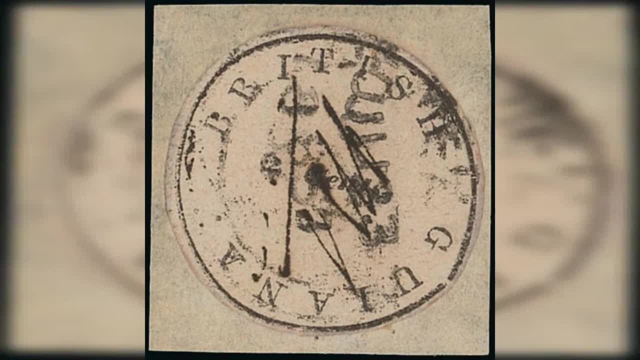 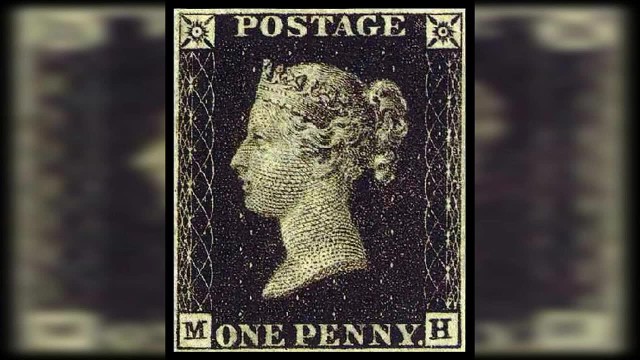 making it the most expensive stamp in the world- Number 15.. Penny Black, Great Britain, 1840,. estimated value: $600,000.. The Penny Black holds a special place in philatelic history as the world's first adhesive postage stamp. It was issued in Great Britain on May 1, 1840, during the reign of Queen. 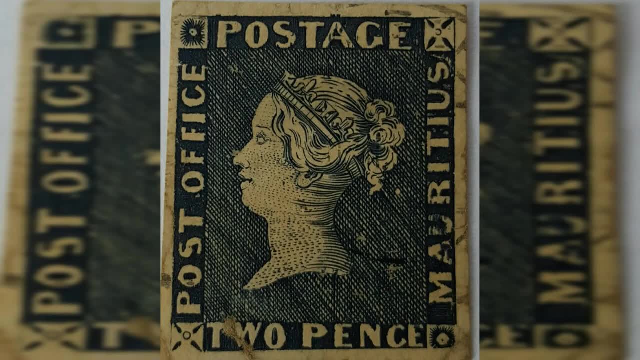 Victoria, Number 14.. Mauritius Post Office: 2P, blue, 1847, estimated value: $600,000.. The Mauritius Post Office stamp is an iconic stamp with a fascinating error in its inscription. The stamp was issued in 1847 and features the words Post Office at the top. 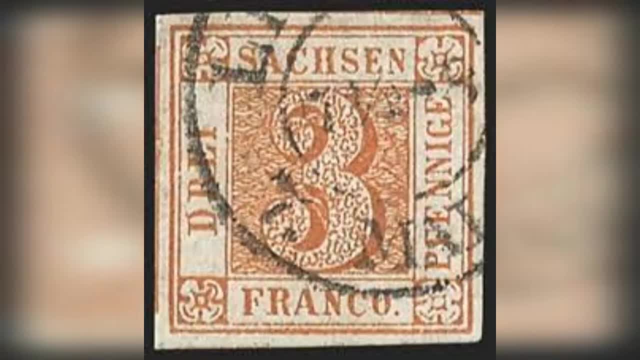 Number 13. Saxony 3PF 1850, estimated value: $630,000.. The Saxony 3PF stamp of 1850 is an important stamp in the postal history of Saxony, a former German state. The 3PF stamp is the first stamp issued in Saxony and played a crucial role in the development of. 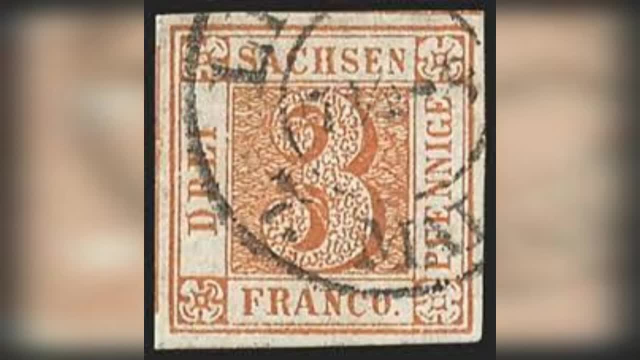 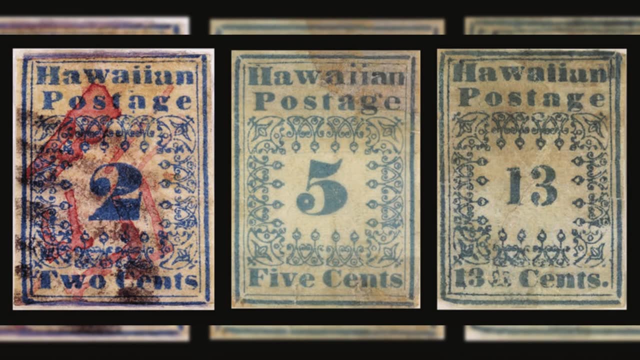 postage systems worldwide. The 3PF stamp is the first adhesive postage stamp ever issued by Saxony Number 12.. Hawaiian Missionaries- Hawaii 1851,. estimated value: $760,000.. The Hawaiian Missionaries are among the first stamps issued by the Kingdom of Hawaii. 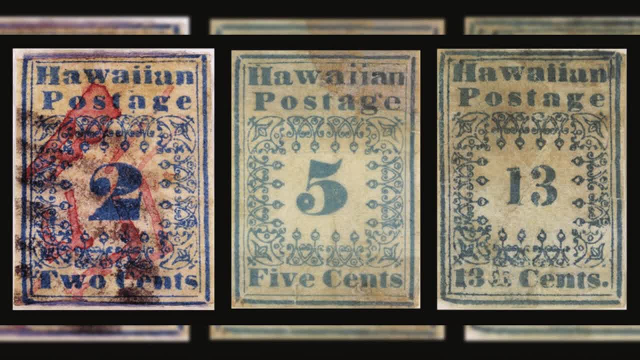 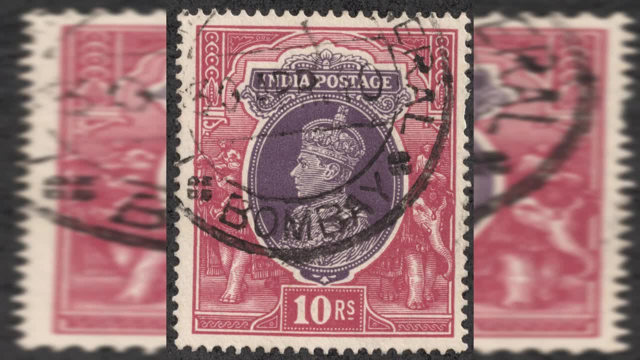 They were introduced in 1851 after Hawaii established its postal system, Number 11.. India 10R. estimated value: $830,000.. The 10R stamp of India is an impressive, high-value stamp issued during the British colonial era. 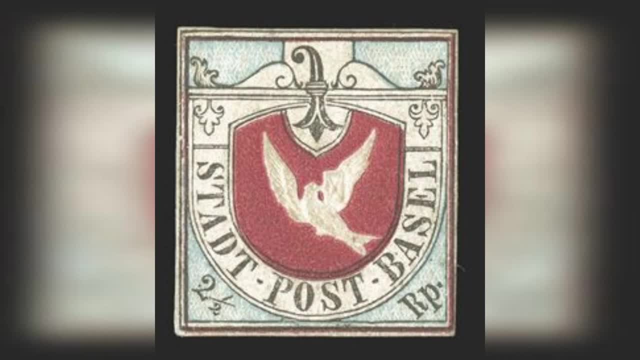 Number 10.. Basel Dove, Switzerland 1845,. estimated value: $1,000,000.. The Basel Dove of the French colonial era was the first stamp issued by the British colonial era. The Barone Dove is a standard stamp of the state, a wildひOLA state historic site, the capital of the city, as well as the Skardina ancient grandmother. 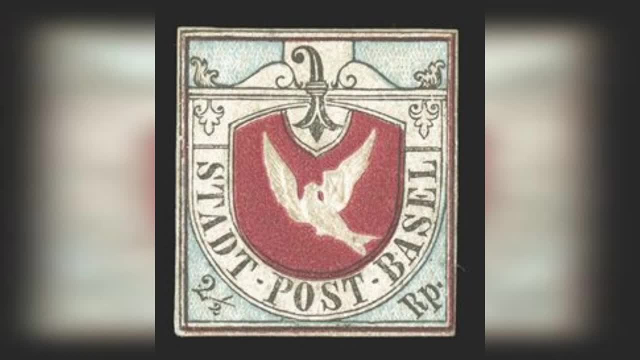 The 2018 Giants display brochure of the model is in Hokkinge, Woahan City, with a traditional inspiration inspired by a Russian saint. Switzerland's first-ever postage stamp, issued by the Canton of Basel. It was released in 1845. 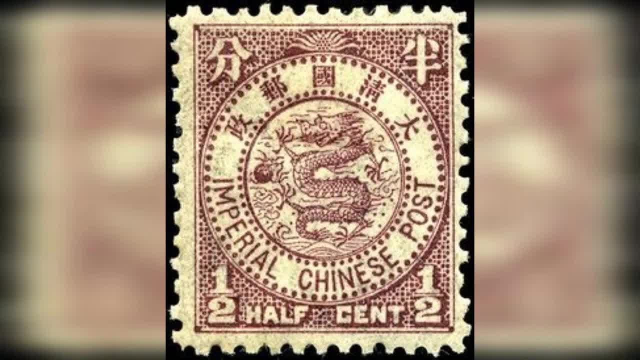 and designed by architect Melchior Berry. Number 9.. Red Mercury, China, 1855,. estimated value: $1 million. The Red Mercury is one of China's earliest stamps, issued in 1855.. Its name comes from the stamp's distinctive red color and features a dragon design. 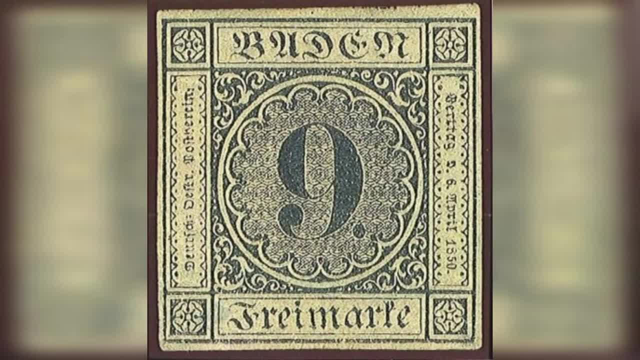 Number 8. Baden 9 Cruiser- Error 1851,. estimated value: $1 million. The Baden 9 Cruiser is a rare stamp from the German state of Baden In 1851, the stamp was mistakenly printed with the denomination 9 Cruiser instead of the correct 6 Cruiser. 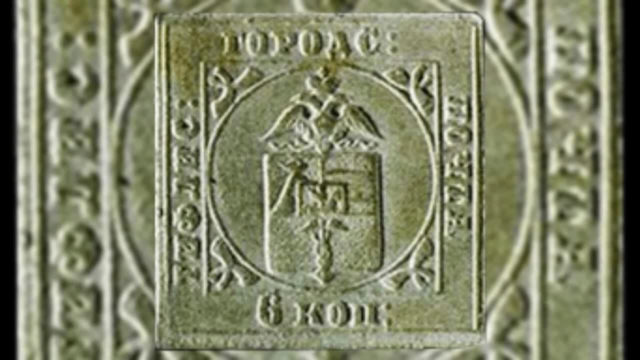 Number 7. Russia- Tiflis Stamp 1857, estimated value: $1 million. The Russia Tiflis Stamp of 1857, estimated value: $1 million. The Russia- Tiflis Stamp of 1857, estimated value: $1 million. 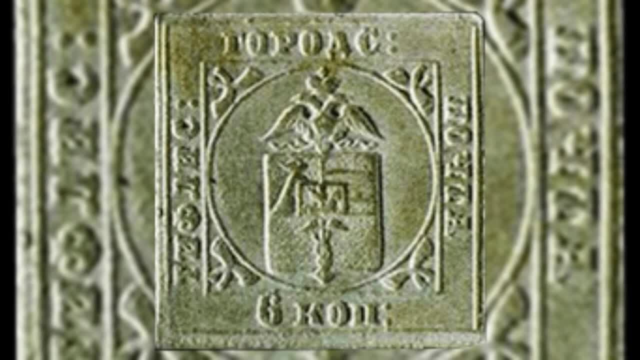 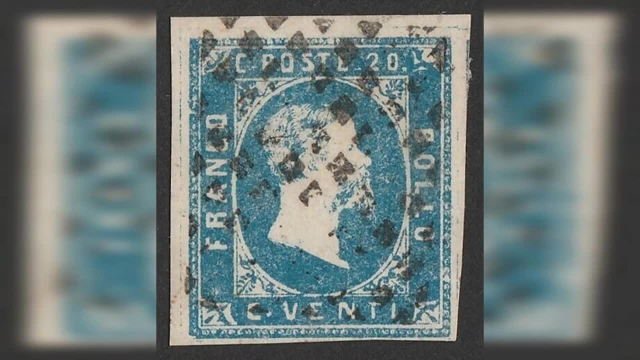 The Russia Tiflis Stamp of 1857, is a remarkable and historically significant stamp issued during the Russian Empire Number 6. Italy- 2 Lira Dark Blue, 1851,. estimated value: $1.5 million. The 2 Lira Dark Blue stamp of Italy is an early and valuable issue of the Kingdom of Sardinia. 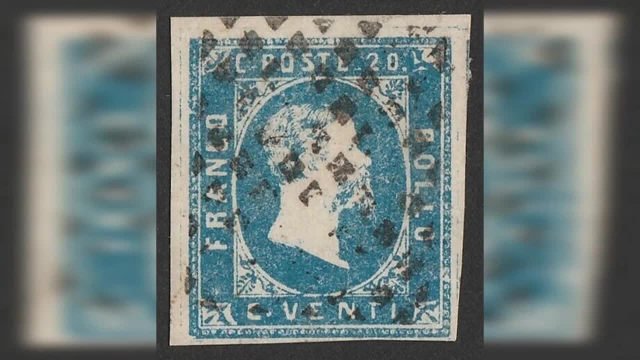 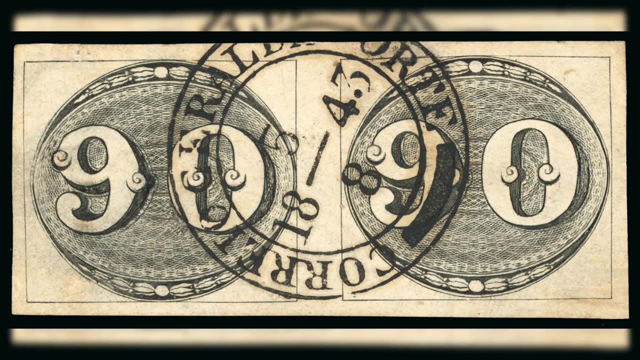 which later became part of unified Italy. It features a portrait of King Charles Albert and was issued in 1851.. Number 5. Brazil Bullseye 1843,. estimated value: $1.5 million. The Brazil Bullseye stamp issued in 1843,. 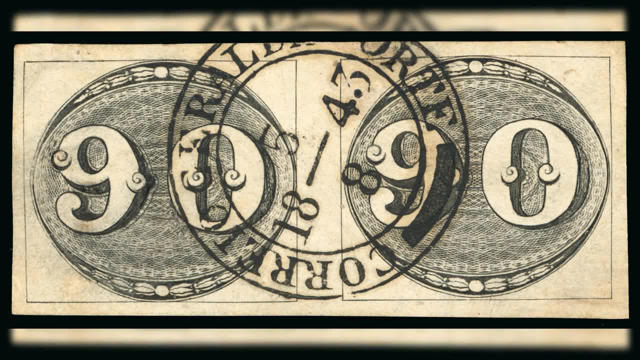 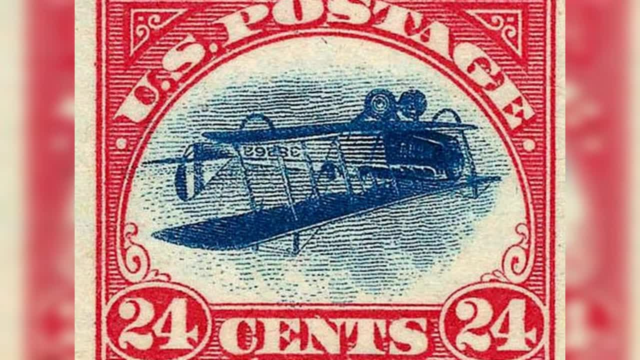 is one of the earliest stamps in South America. It features a central bullseye design with various denominations surrounding it. Number 4. Inverted Jenny, USA 1918, estimated value: $1.6 million. The Inverted Jenny is an iconic stamp from the United States. 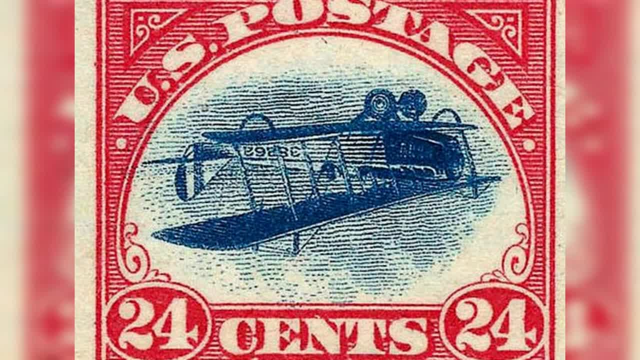 issued in 1915.. Number 6. Brazil Bullseye 1843, estimated value: $1.5 million. The Brazil Bullseye 1853, estimated value: $1.6 million. It features a Curtis JN4 biplane known as Jenny.